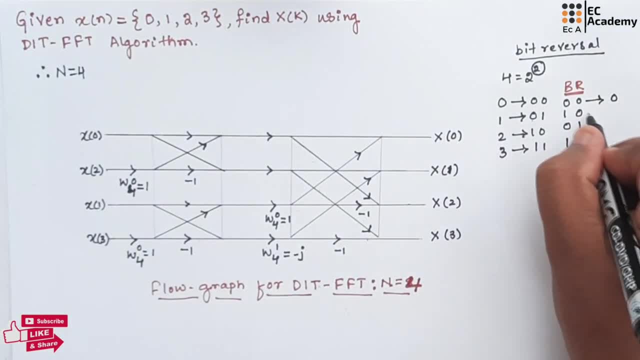 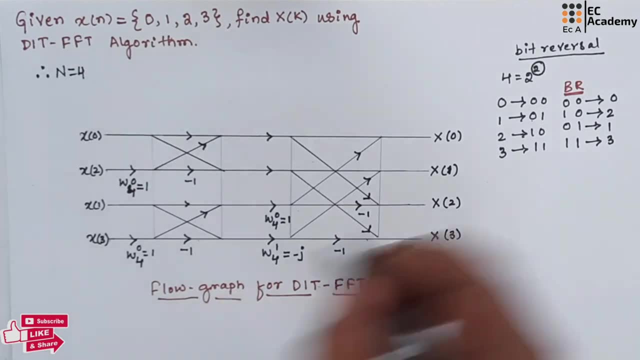 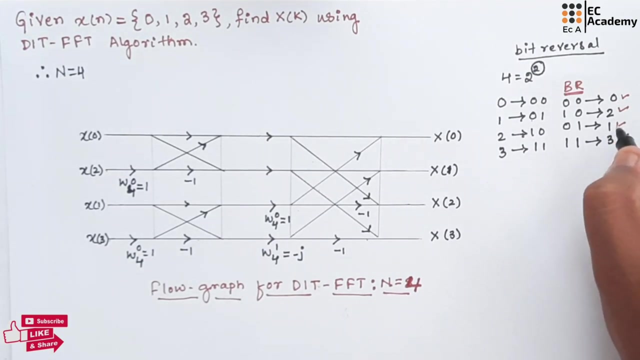 as 1: 1 itself. 0: 0 is 0,, 1, 0 is 2,, 0- 1 is 1,, 1: 1 is 3.. Now you can use these values at the input, So you can take first value as x of 0,, second value is x of 2, third value: 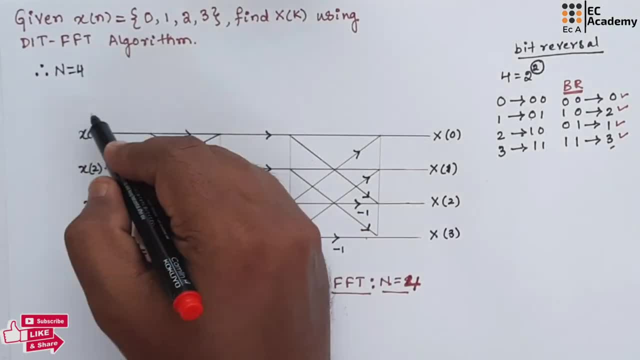 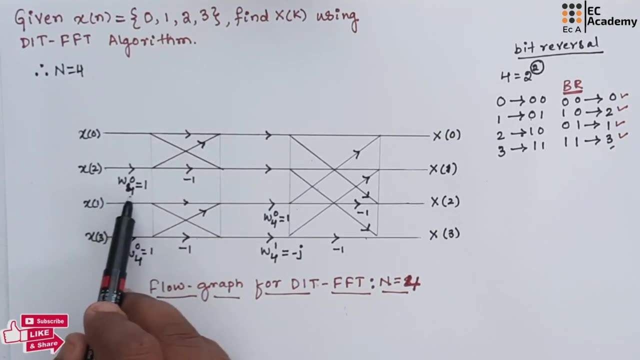 is x of 1 and fourth value is x of 3.. So you will not be having any confusions. So in this flow graph you need to remember: w 4 to the power of 0 is 1 and also w 4 to 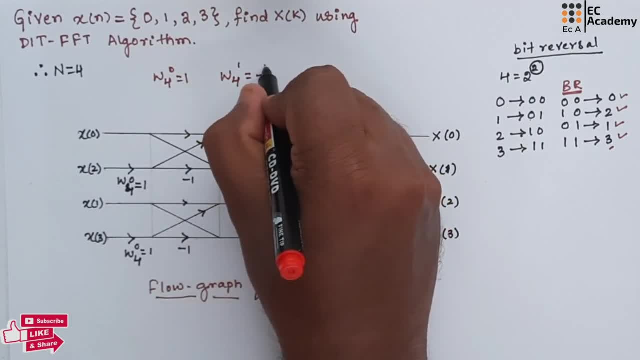 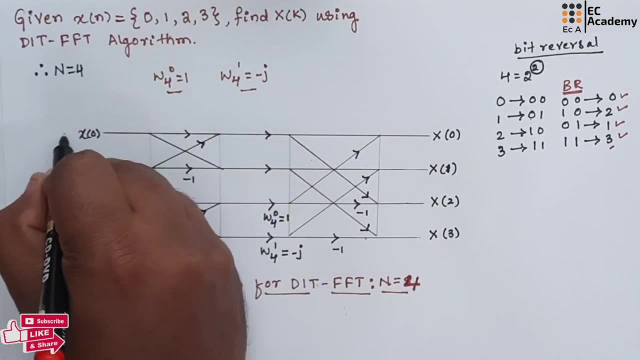 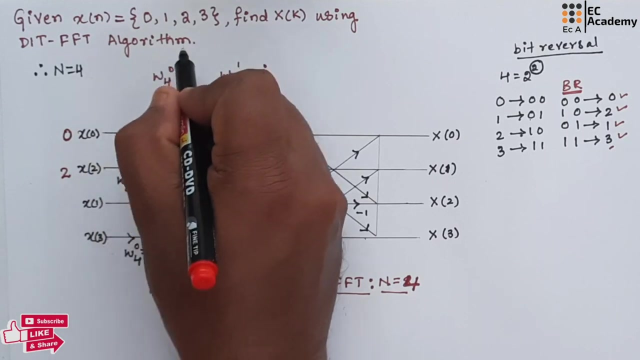 the power of 1 is minus j. So these two values you can remember so that we can use that for calculations. So x of 0 is 0,, x of 2 is 2, x of 1 is 1 and x of 3 is 2.. 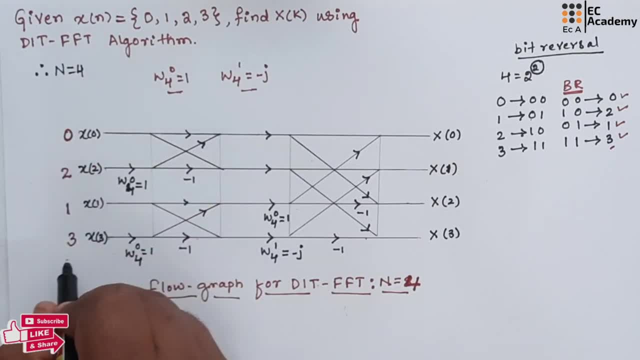 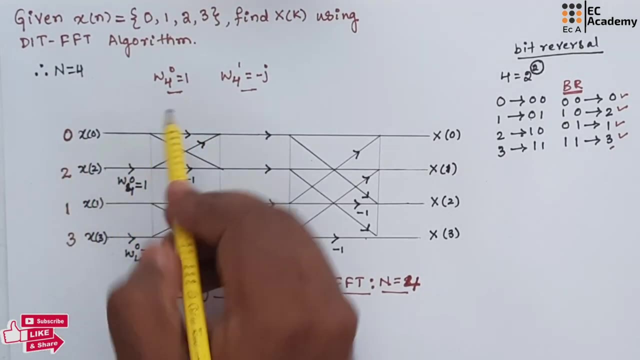 is 3.. So these are the inputs we need to give. After writing the input, you just need to follow the arrow marks. So just follow the arrow marks so that you can get the value. Now let us start from this point. It is on this line, So it is 0.. For this you are having. 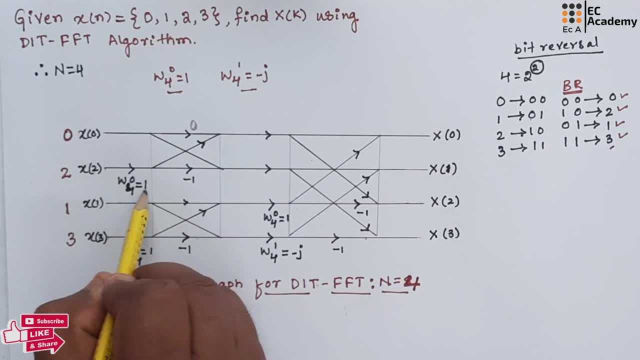 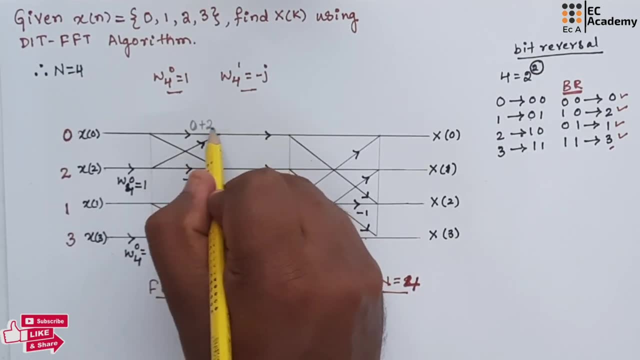 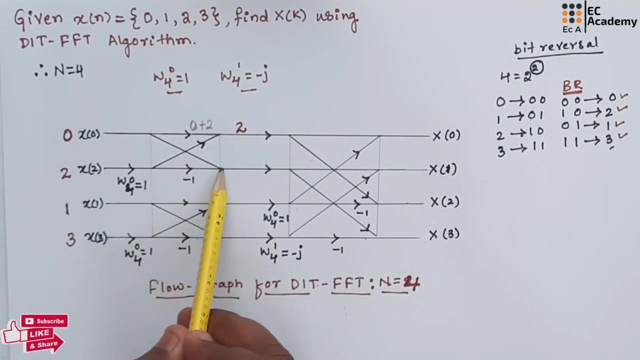 this connection. So it will be 2 into 1 on this line, So 0 plus 2.. So at this point you are getting the answer as 2.. Now we need to find at this point what is the answer. So it is 0 plus 2 into minus 1.. It is minus 2.. 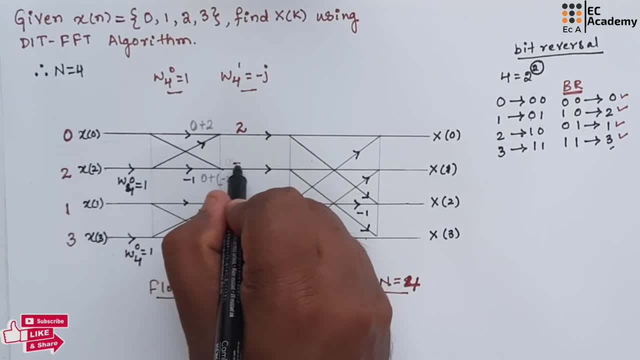 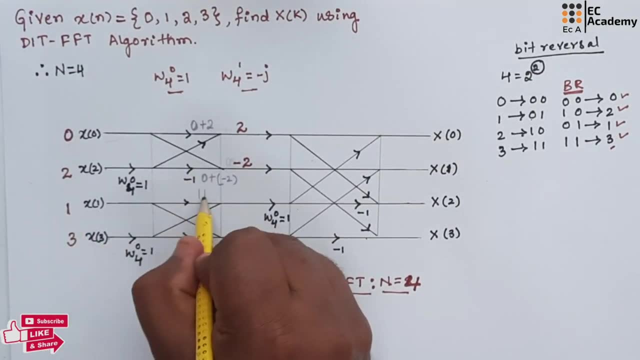 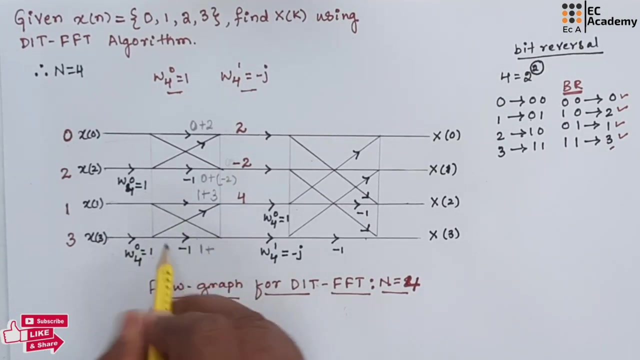 So it will be minus 2.. In the same way, let us calculate for x of 1.. So it is 1 plus 3 into 1, it is 3.. So you will get answer as 4.. Again, on this line, 1 plus on this line it will. 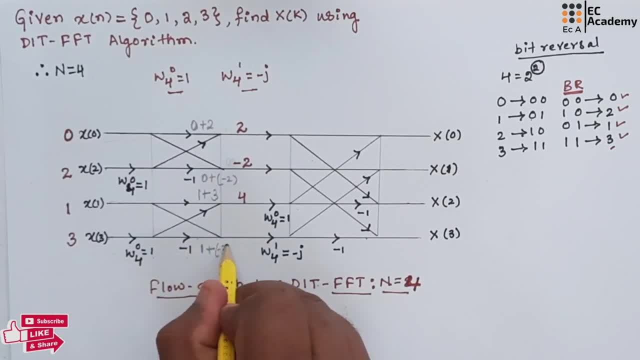 be 3 into minus 1, it will be minus 3.. So 1 minus 3, it is minus 2.. So we got the intermediate answers. after performing the first stage, For the next stage you need to take this as input and you need to calculate Now on. 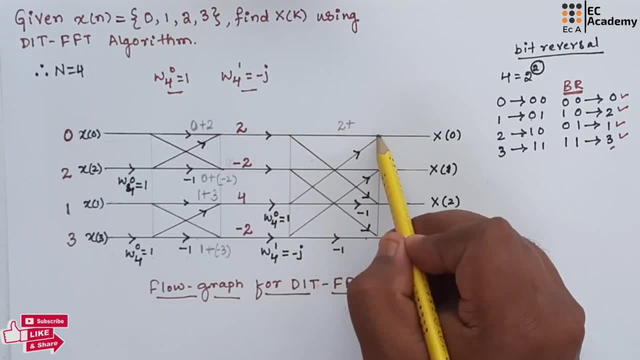 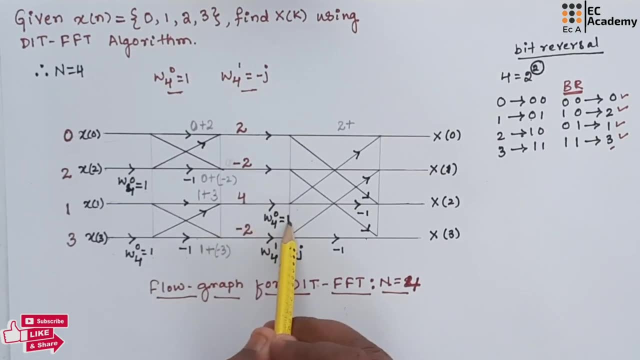 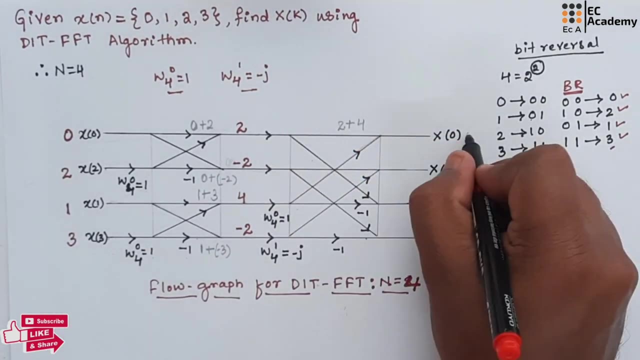 this line it is 2 plus. for this point you are having the arrow mark here, So you can take the input from this point 4 into 1 minus 3.. So 2 plus 4 into 1, it is 4.. So 2 plus 4, it is 6.. So x of 0 is 6.. Now on this line. 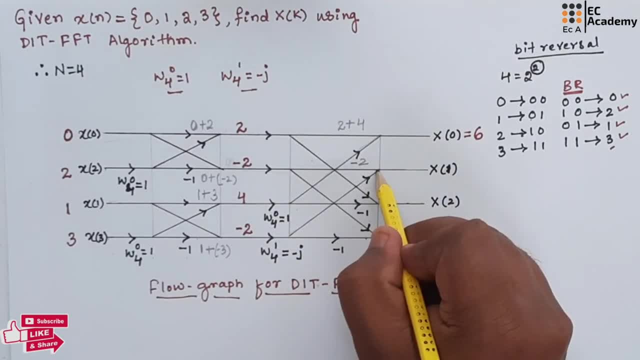 it is minus 2.. For this point you are getting the input from this line. So it is minus 2 into minus j. it is plus 2j. So it is plus 2j. So the answer for x of 1 minus 3 into: 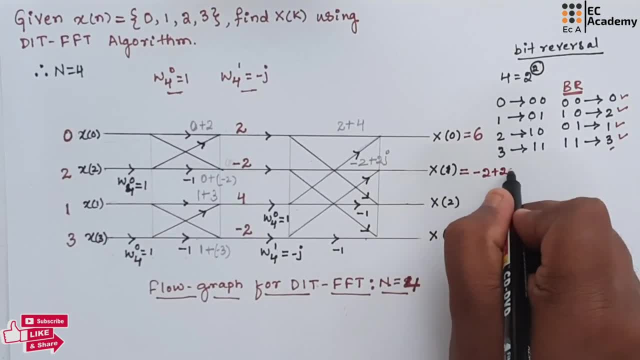 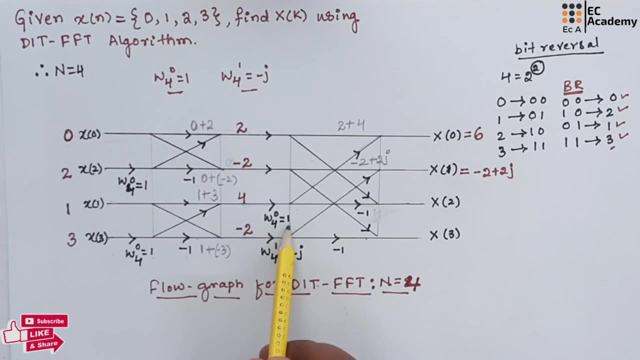 minus 1 is minus 2 plus 2j. On this line you are having the input as 4, 4 into 1, it is 4, 4 into minus 1.. Again, you are having minus 1 here. it will be minus 4.. At this, 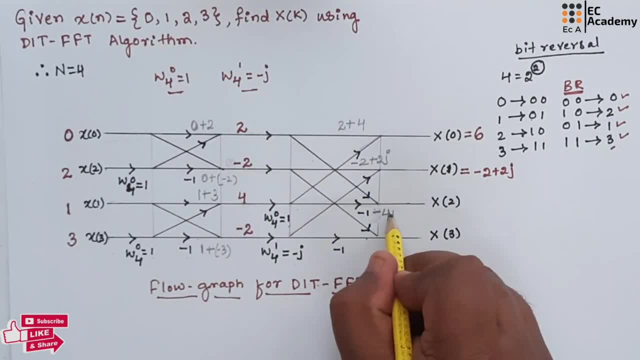 point you are getting the input from this line. it is 2 plus 2.. So minus 4 plus 2, it is minus 2.. Now, on this line, you are getting the input as minus 2.. So minus 2 plus 2 into. 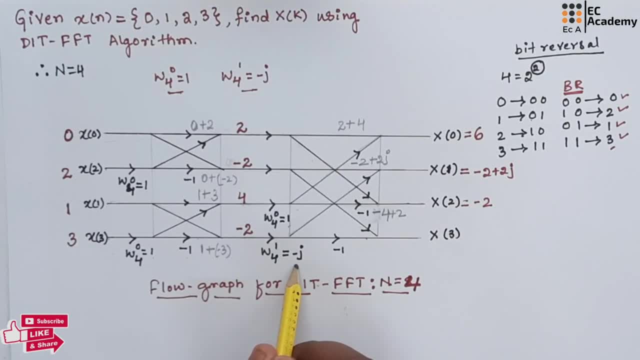 2 into minus j, it is 2 j into minus 1, it is minus 2 j. At this point you are getting the input on this line. So it is minus 2.. So minus 2 j plus of minus 2.. So the value. 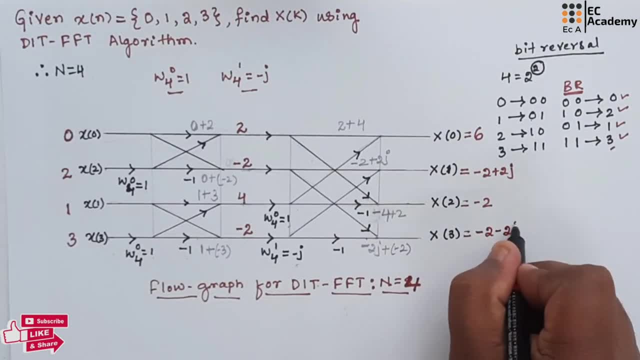 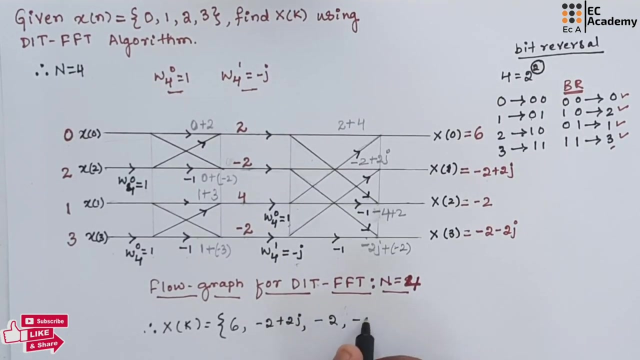 is minus 2 minus 2 j, So this is the DFT value after calculation using DIT FFT. So finally we can write: x of k is equal to: so it is 6 minus 2 plus 2 j minus 2 and minus. 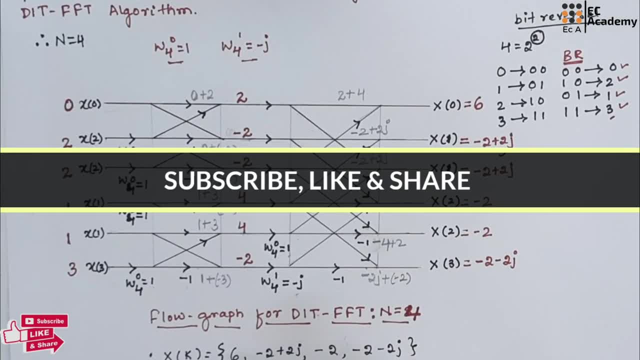 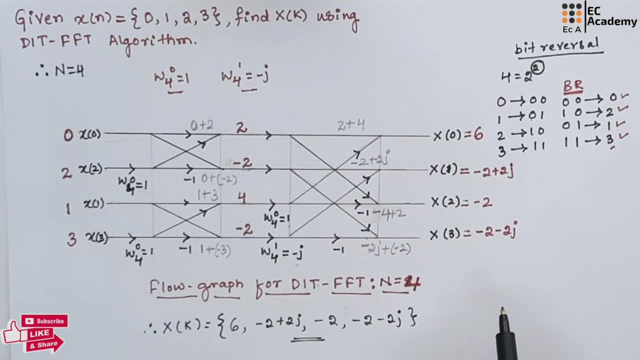 2 minus 2. j is about the problem on DIT. FFT for n is equal to 4.. Hope you have understood this topic. Thank you.